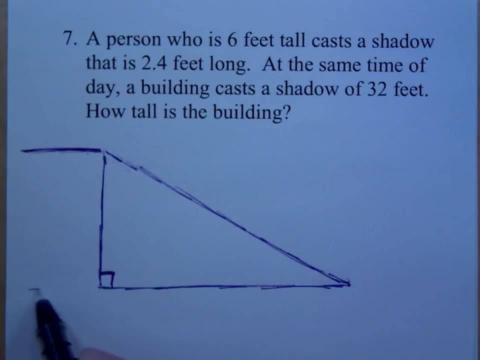 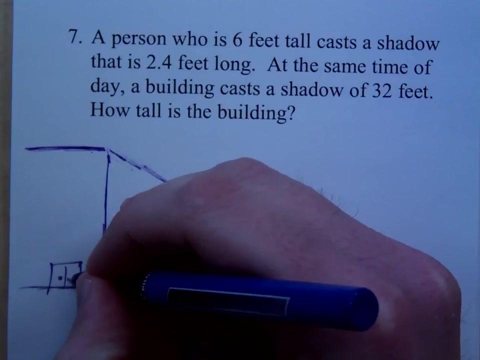 If this is your building over here, and here is the length of his shadow. Are you with me on that picture? I'm sorry here let me do this. Here's the doors, And of course, all the windows have to look like that, right. 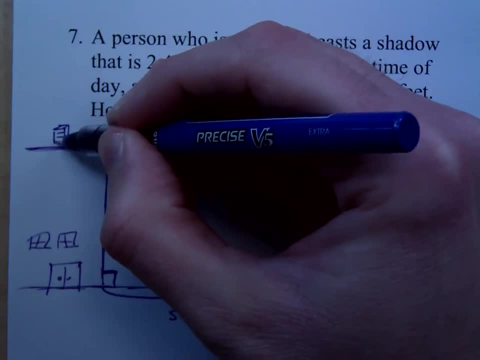 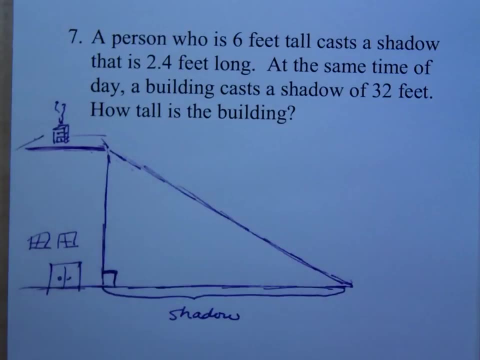 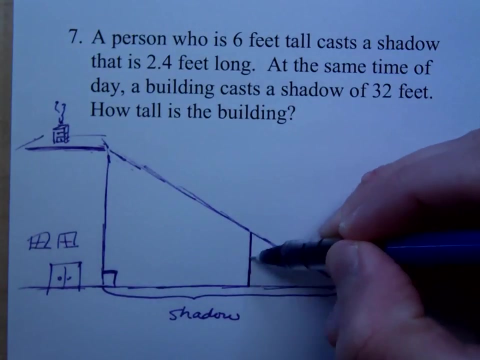 Maybe he's got a little chimney up here, because, after all, that's what all buildings have. So anyway, there's your building Now with a triangle. no matter where you are, if you draw something like this, it's going to be proportional. 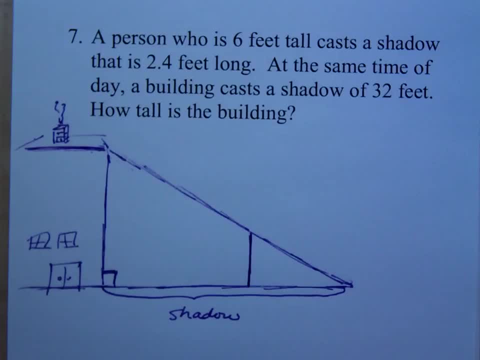 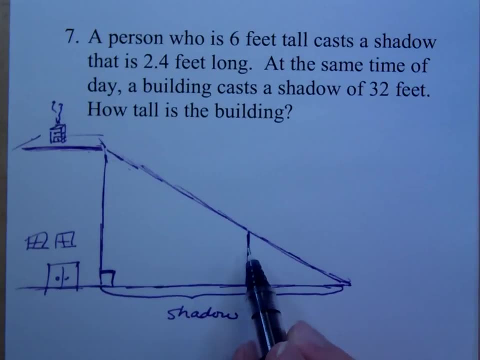 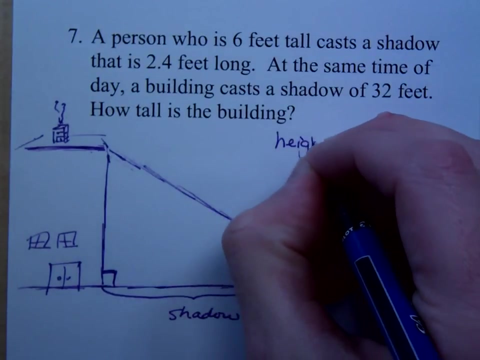 We talked about. If you remember geometry, hopefully you remember similar triangles. That means that the height to the length is going to be in proportion to the height to the length. So we could do this. We can say the height of the object to the length of the shadow. 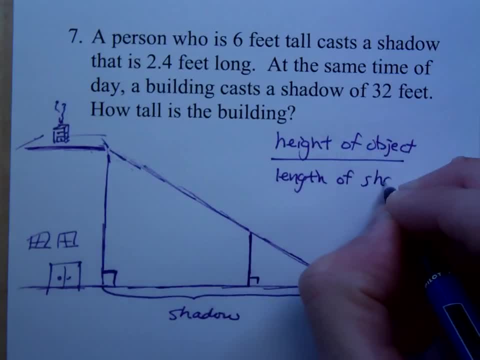 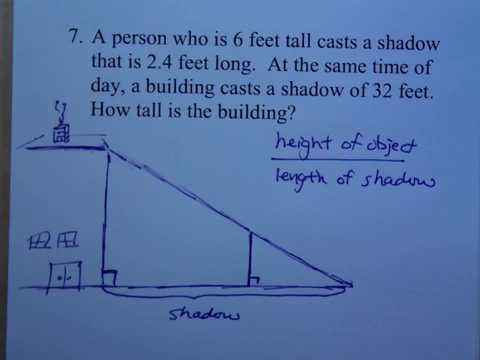 That's the framework that we're going to be using here, Because- think about this, If you were outside on a sunny day- the taller the object is, the longer its shadow is right, So that's proportions. So let's look at it this way. 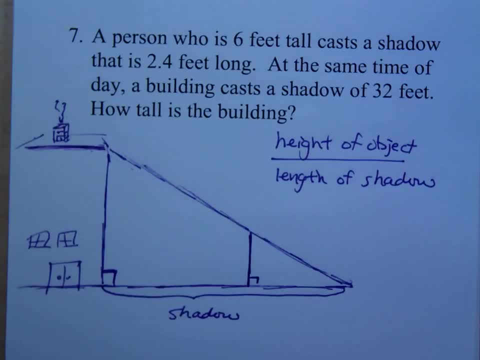 Do we know something about the height of an object? What do we know? Six feet tall? Six feet tall measures, how long? 2.4 feet, 2.4 feet for the shadow right. So the height to the length. 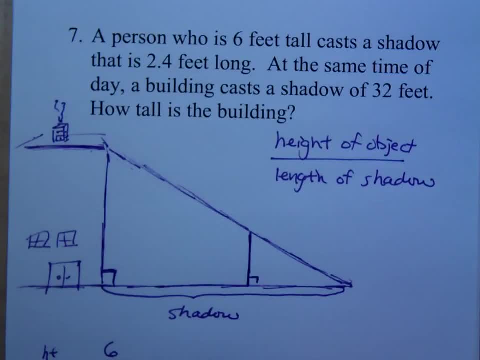 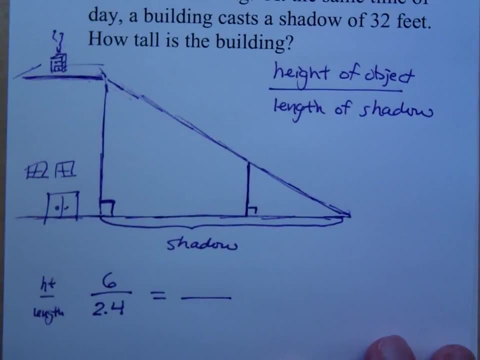 So what's the height of the building? X, 32.. Ooh, Is it X or is it 32?? Oh, sorry guys, It's unknown, because it says how tall is the building. I don't know how tall it is, but I do know that the length of the shadow is what. 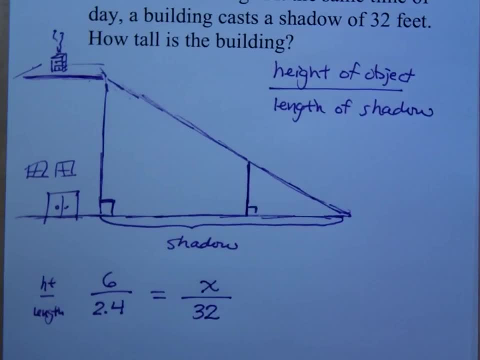 I do know that that's 32.. Now look at this. That shadow is considerably longer than the shadow of the man or person. It doesn't say man, the person, Okay, So I would expect that the height of the building would be a lot taller than the height of the person, right?